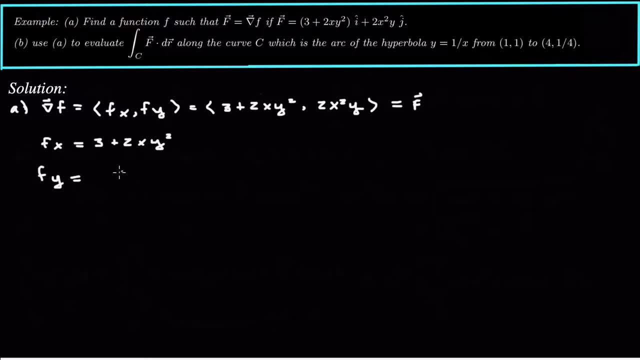 And f sub y should be equal to 2x squared y. So if I integrate those with respect to their correspondingDerivatives, and then we have to separate those both and then we have variables, I should get f of x- y. So f of x- y will be equal to in the first case. 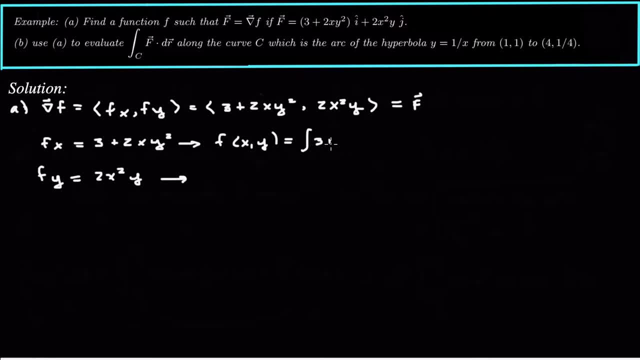 the integral of 3 plus 2xy squared dx, which we could say is just integrating with respect to x. So it's 3x plus x squared y, or sorry, x squared y squared plus maybe something that only depends on y, so we'll call that g of y, So maybe something that only depends. 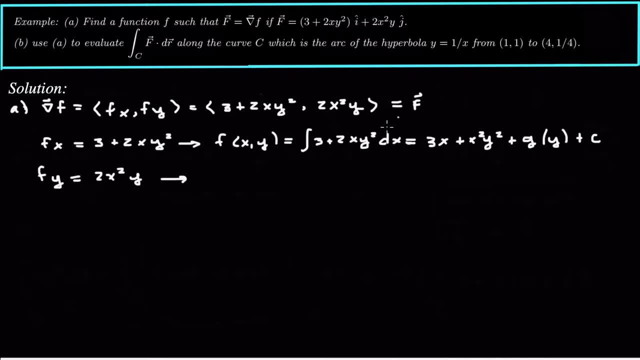 on y plus a constant. we'll stick that in there explicitly like that. The second one, f sub y, equals 2x squared y. if I integrate that with respect to y, I get f of x- y, which is the integral of 3y squared dx y. So if I integrate that with respect to y, I get: 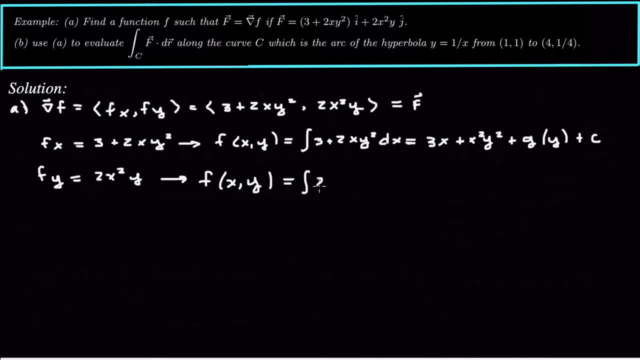 f of x- y, which is the integral of 3y squared dx- y. So if I integrate that with respect to y, I get f of x- y, which is the same function should be equal to the integral of 2x squared y- dy. But now I'm integrating with respect to y and I would get x squared. 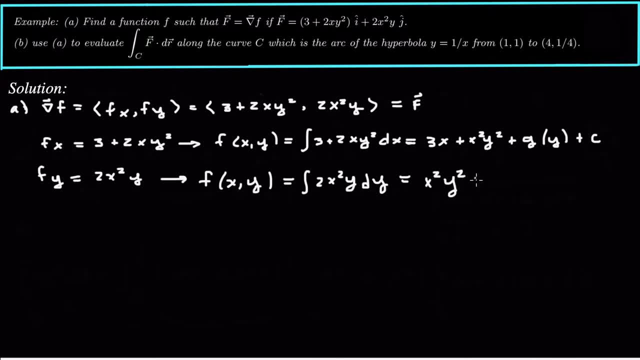 y squared plus maybe we'll say some function that only depends on x plus a constant. Now why do I add these functions that maybe only depend on y or only depend on x? Well, in this function that's just dependent on y, and you differentiate that with respect to. 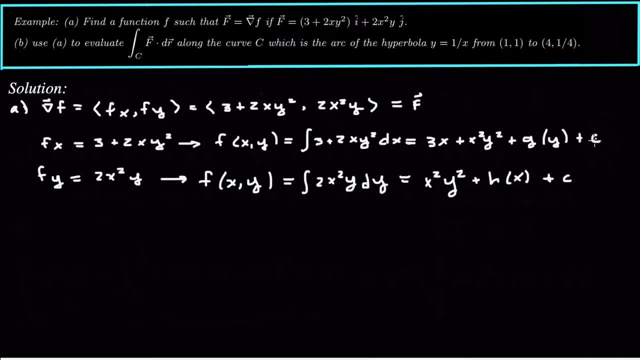 x. it's going to go away, It's going to be zero. Same thing with this constant. Differentiating a constant, we get zero. So these two terms would just go to zero when I differentiate. So if I differentiate with respect to x, I get 3 plus 2xy squared, which is exactly. 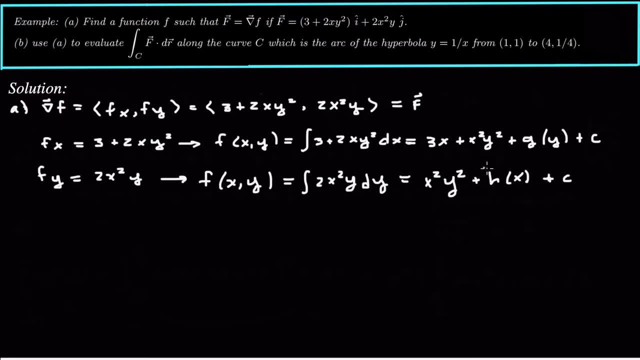 what I want in my gradient. Now the same thing in the y, or the second part of the function f of x. y equals x squared, y squared plus h of x plus a constant. Then I differentiate this with respect to y. this constant goes away and this h of x would go away If I 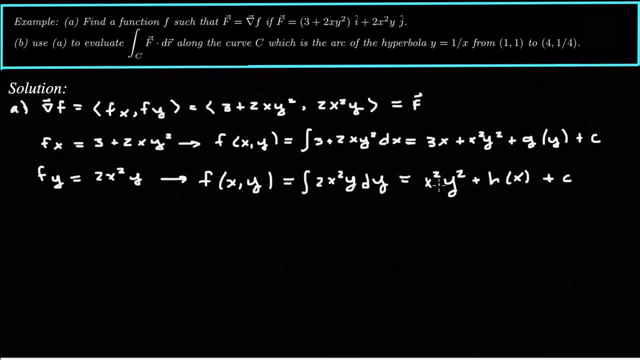 look and compare these two functions. this matches. but then I have a function of only x right here. so h of x is equal to 3x and g of y. I don't have anything that depends only on y. so I'll say g of y is just zero, and then I can say that my function f of x. 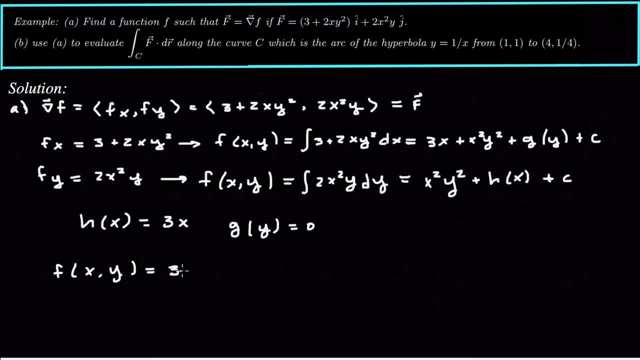 is equal to 3x plus x squared, y squared plus maybe a constant c, And that is good enough for part a, because we don't necessarily need to know what the constant is. If we were given some point that we could plug in, we could figure out what the constant is. but 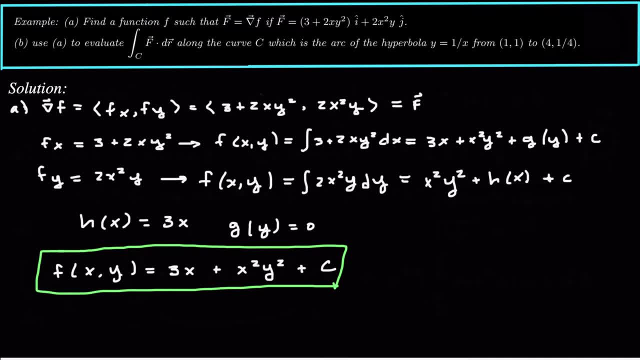 we don't have that, so we'll just stop right there and say that's our function, 3x plus x squared, y squared, And then we want to use that. We want to use part b to evaluate the line integral. so let's look at part b. So for 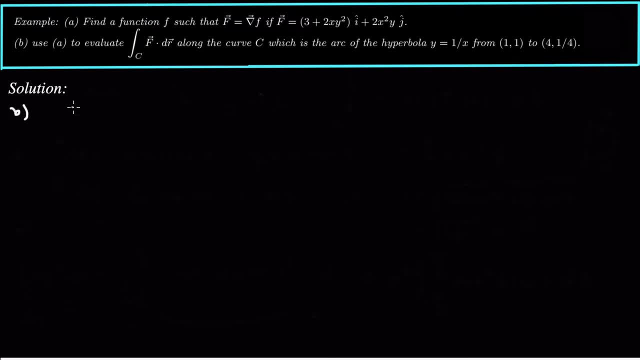 part b. the main thing to remember is that the integral over the curve c of a gradient, so a conservative vector field, is just the vector field, the potential function evaluated at the second point Minus the potential function evaluated at the first point. So this is what we call path. 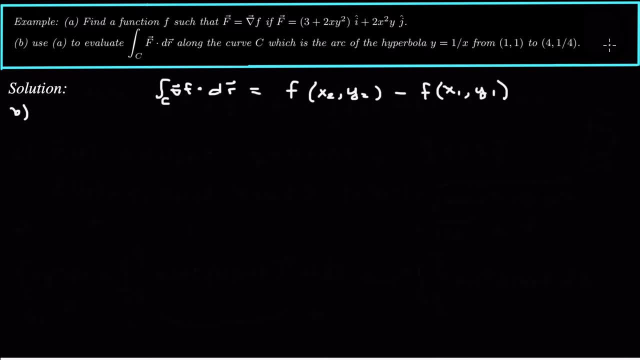 independence. It doesn't matter what path you take to get between these two points. what matters is the points themselves. so a conservative field. that's the key. So we're going to say that the integral over the curve c, f, dot, dr is equal to the line integral. 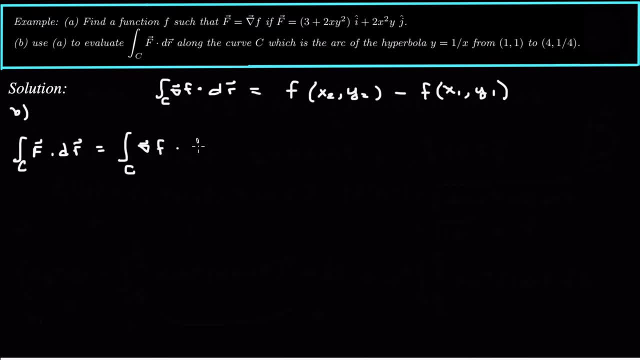 of the gradient of little f which we just found, dot dr, because we've said that f equals gradient of little f. Now, by the fundamental theorem of calculus for line integrals, we just say that this is going to be f of x2 comma y2 minus f of x1 comma y1.. Now what?